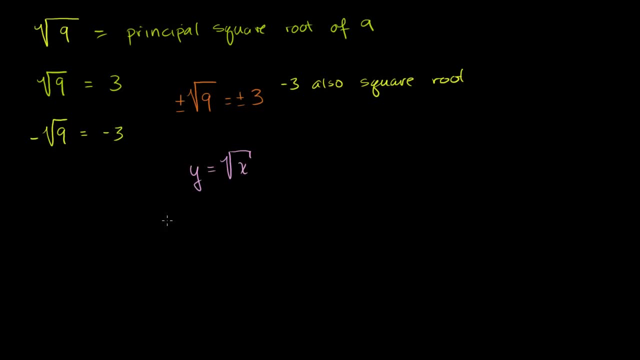 principal square root And see how it relates to the function. y is equal to x- Let me write it over here because I'll work on it- See how it relates to: y is equal to x squared And then, if we have some time, we'll shift them around a. 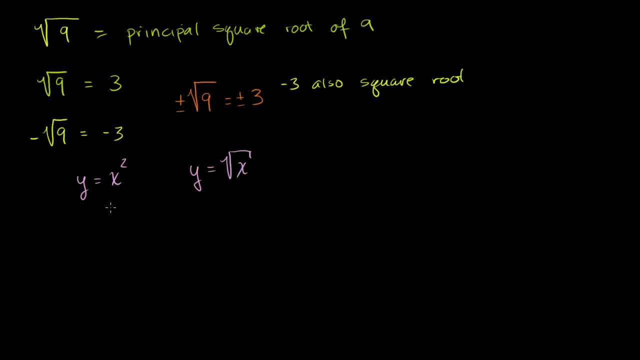 little bit and get a better understanding of what causes these functions to shift up, down or left and right. So let's make a little value table before we get out our graphing calculator. So this is for y is equal to x. This is for y is equal to x squared. 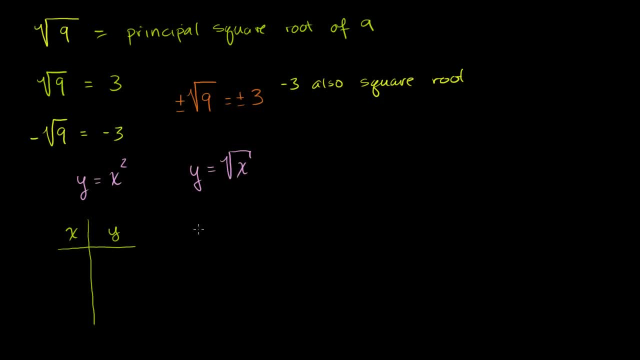 So we have x and y values, And this is y is equal to the square root of x, And once again we have x and y values right there. So let me just pick some arbitrary x values right here and I'll stay in the positive x domain. 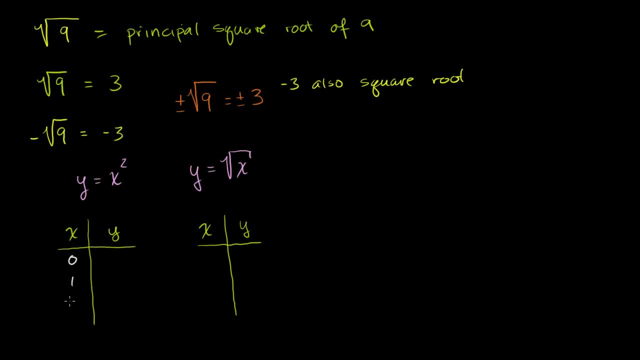 So let's say x is equal to 0, 1.. Let me make it color coded: When x is equal to 0, what's y going to be equal to? Well, y is x squared, so 0 squared is 0.. 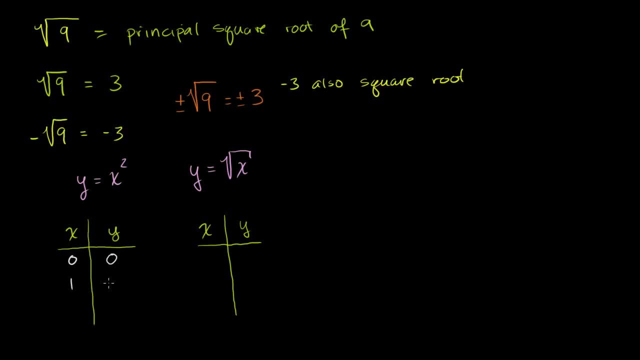 When x is 1, y is 1, squared, which is 1.. When x is 2, y is 2, squared, which is 4.. When x is 3, y is 3 squared, which is 9.. 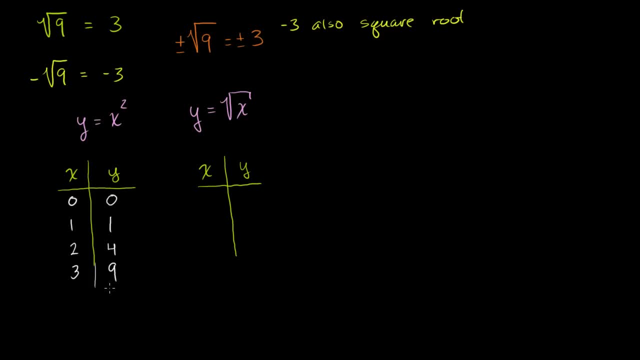 We've seen this before and I could keep going. Maybe I'll add a little. Let me add 4 here. So when x is 4, y is 4 squared or 16.. We've seen all of this. We've graphed our parabolas. 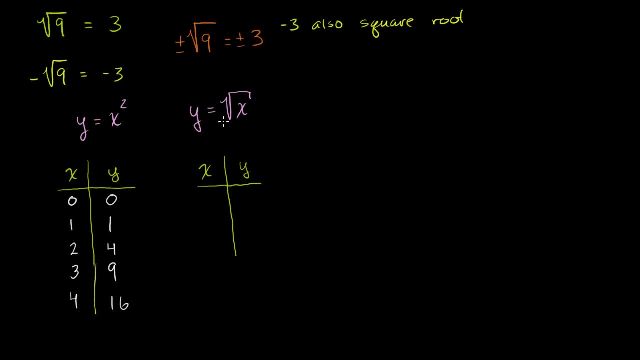 This is all a bit of review. Now let's see what happens When y is equal to the principal square root of x. Let's see what happens, And I'm going to pick some x values on purpose, just to make it interesting. 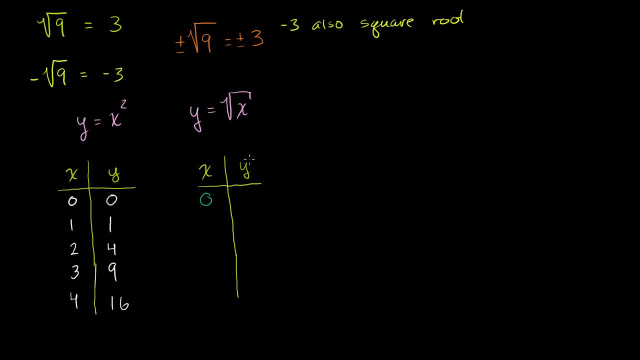 When x is equal to 0, what's y going to be equal to The principal square root of 0, what's 0?? 0 squared is 0.. When x is equal to 1, the principal square root of x of 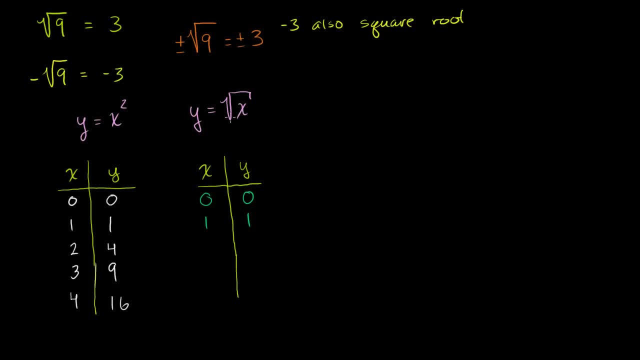 1, is just positive 1.. It has another square root, that's negative 1, but we don't have a positive or negative written here, We just have the principal square root. When x is 4,, what is y? Well, the principal square root of 4 is positive 2.. 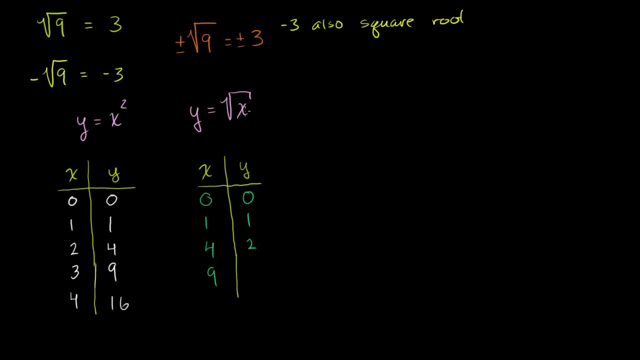 When x is equal to 9, what's y? When x is equal to 9,, the principal square root of 9 is 3.. Finally, when x is equal to 16, the principal square root of 16 is 4.. 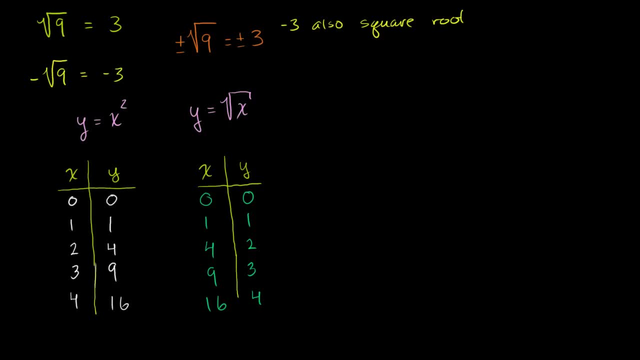 So I think you already see how these two are related. We've essentially just swapped the x's and the y's, right? Well, these are the same x's and y's, but here you have: x is equal to y is 4.. 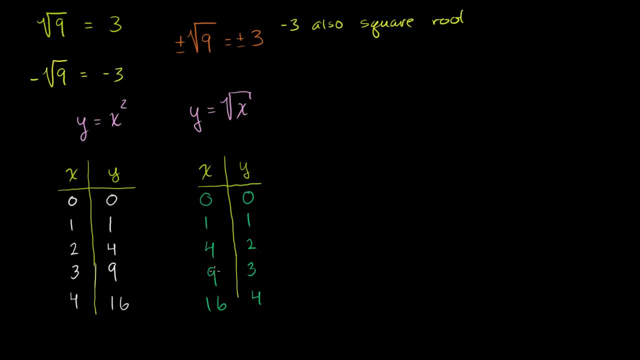 Here, x is 4, y is 2.. 3 comma 9, 9 comma 3,, 4 comma 16, 16 comma 4.. That makes complete sense. If you were to square both sides of this equation, you 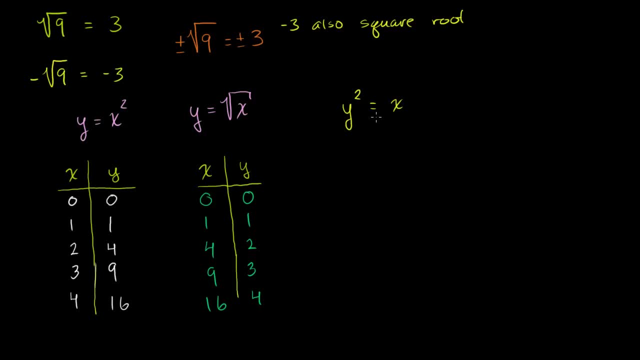 would get y squared is equal to x, right there. Of course you would want to restrict the domain of y to positive y's. This can only take on positive y's, on positive values, because this is a principal square root. but the general idea is we just swapped the x's and y's. 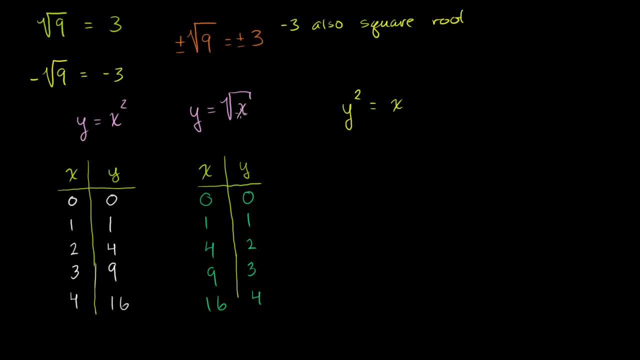 between this function and this function right here, if you assume a domain of positive x's and positive y's. Now let's see what the graphs look like, And I think you might already have a guess of what. Let me just graph them here. 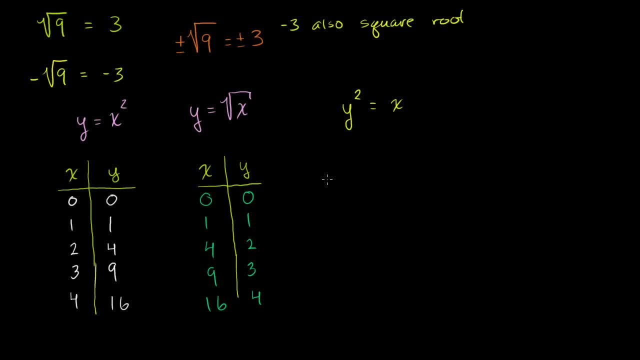 Let me do them by hand, because I think that's instructive sometimes, before you take out the graphing calculator. So I'm just going to stay in the first quadrant here, In the first quadrant. So let me graph this first. So we have the point 0, 0, the point 1, comma 1, the point 2. 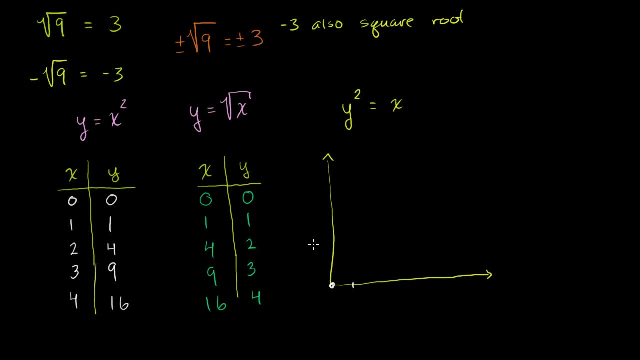 comma 2, which I'm going to have to do it a little bit smaller than that. Let me mark This is 1,, 2, 3.. Actually, let me do it like this. Let me go 1, 2,, 3, 4,, 5, 6, 7,, 8,, 9,, 10,, 11,, 12,, 13,, 14,, 15,. 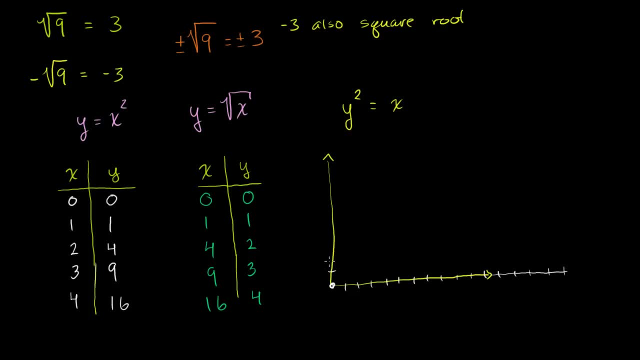 16.. That's about how far I have to go. And that's about how far I have to go. I have 1, 2,, 3,, 4,, 5,, 6,, 7,, 8,, 9,, 10,, 11,, 12,, 13,, 14,, 15,, 16.. 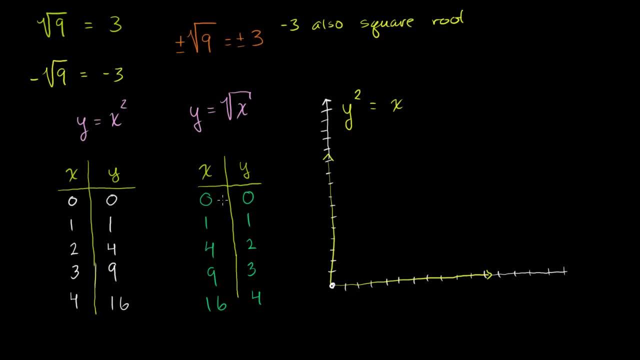 That's about how far I have to go in that direction as well. Now let's graph it. So we have 0, 0, 1, 1, 2 comma 1, 2, 3, 4, 2 comma 4 right. 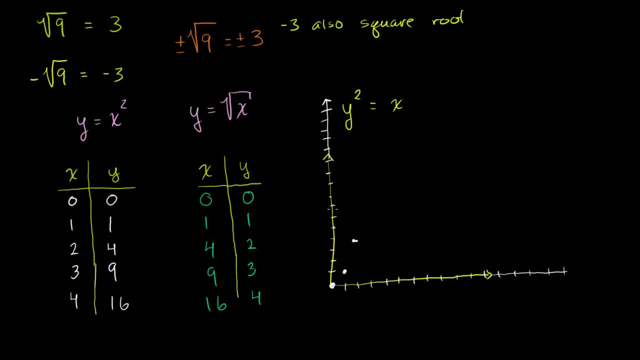 there 3 comma 9,, 3 comma 5,, 6,, 7,, 8,, 9,, 3 comma 9.. That is right about there. And then we have 4 comma 16.. 4 comma 16 is going to be right about there. 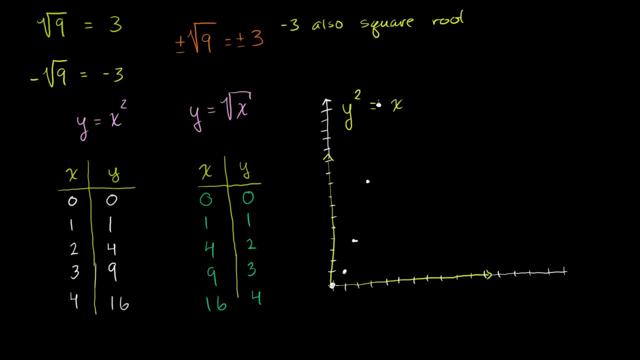 So the graph of y is equal to x squared. We've seen this before. It's going to look something like this: We're just graphing it in the positive quadrant, So we get this upward opening u just like that. Now let's graph: y is equal to the principal square root of x. 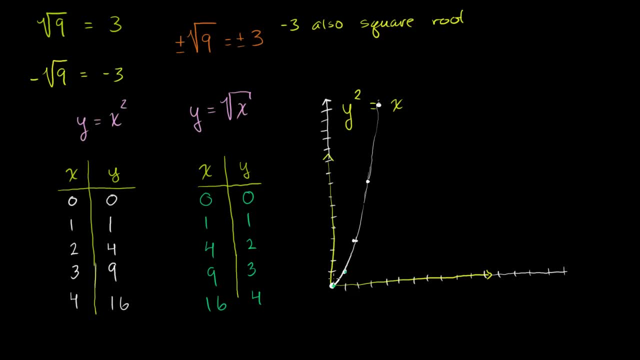 So here, once again, we have 0,, 0.. We have 1 comma 1.. We have 4 comma 2.. 1,, 2,, 3,, 4 comma 2.. We have 9 comma 3.. 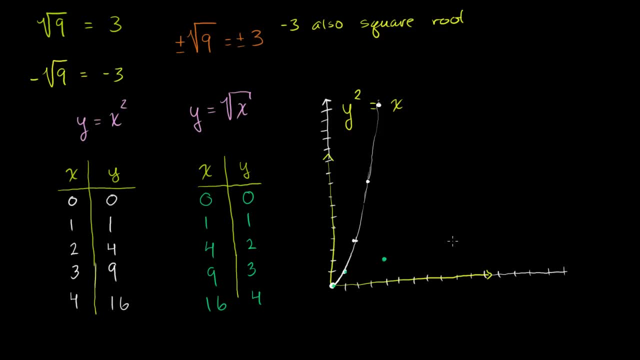 5,, 6,, 7,, 8, 9 comma 3 right about there, And we have 16 comma 4.. 16 comma 4 is right about there. So this graph looks like that. So notice, they look like they're kind of flipped around. 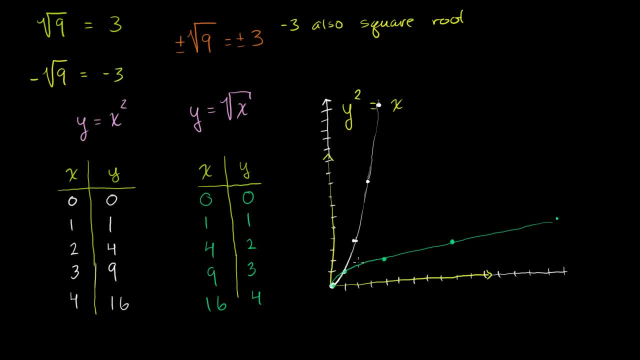 the axes. This one opens along the y-axis, This one opens along the x-axis. And once again it makes complete sense because we've swapped the x's and the y's, especially if you just consider the first quadrant, And actually these are symmetric. around the line y is. 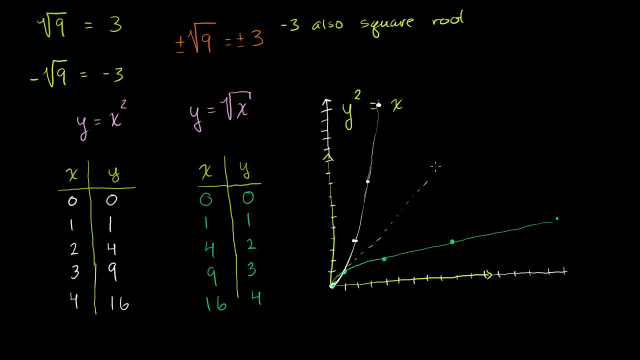 equal to x, And we'll talk about things like inverses in the future that are symmetric around the line. y is equal to x, And we can graph this better on a regular graphing calculator. I found this on the web. I just did a quick web search. 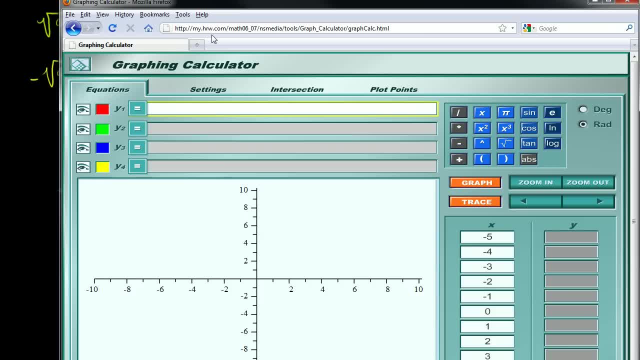 I want to give proper credit to the people whose resource I'm using. So this is myhrwcom slash math06.. You could pause this video and hopefully you should be able to read this, especially if you're looking at an HD. 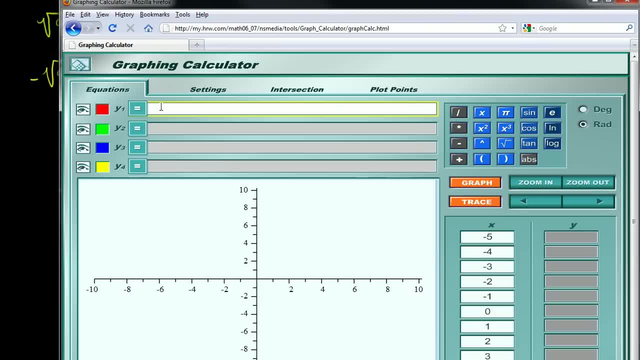 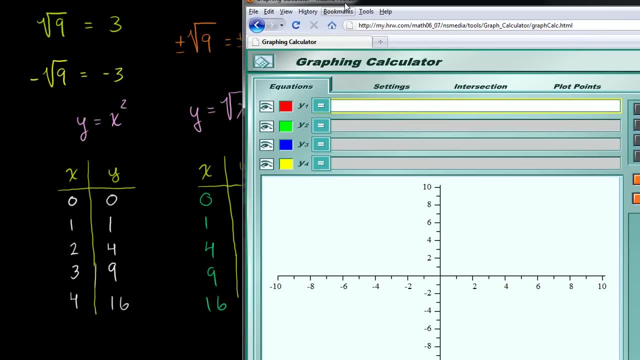 But let's graph these different things, Let's graph it a little bit cleaner than what I can do by hand, And actually let me have some of what I wrote there, OK, So let's first just graph: y is equal to x. 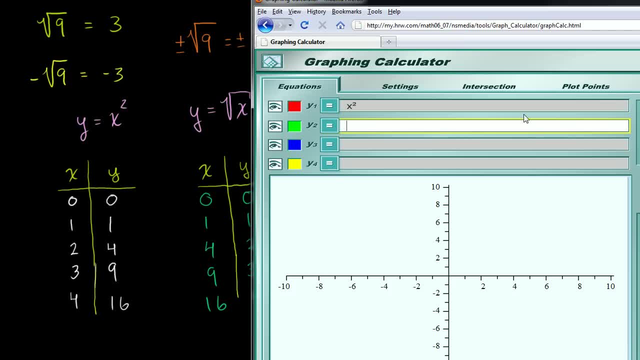 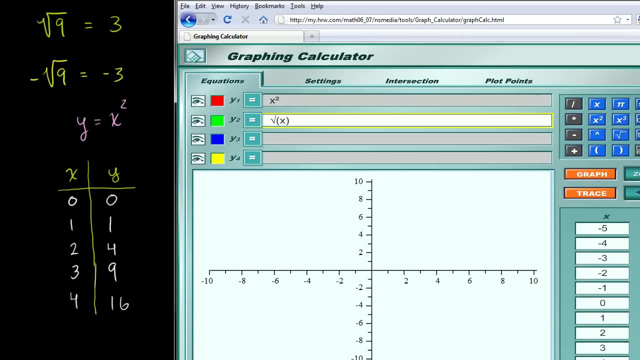 And then in green, let me graph: y is equal to the square root of x. There's some buttons here on the right, just so you know what I'm doing. I have some buttons here on the right. It's squared and the radical sign and all of that. 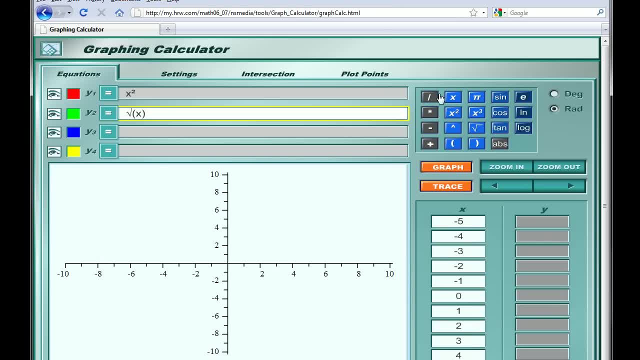 But I want you to just focus on this, So let me just graph those. So first it did x squared and then it did the square root of x And look, if you just focus on the first quadrant right here, you see that you get the exact same result that I got. 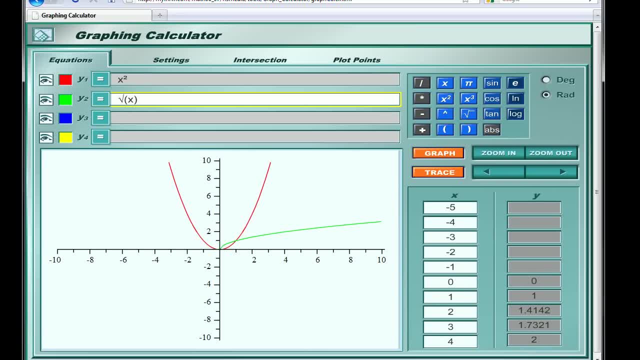 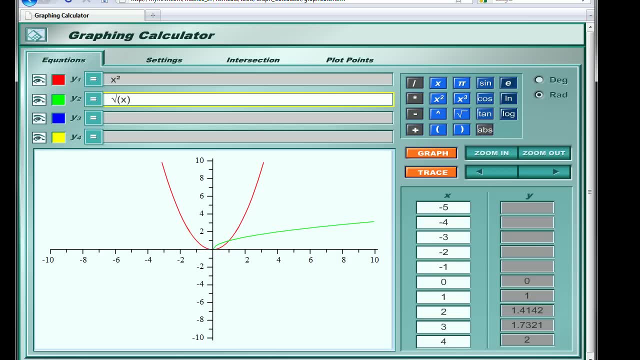 It's over there, although mine is messier Now, just for fun, and I really didn't do this yet with the regular quadratics, Let's see what happens, what we need to do to shift the different graphs. So, with x squared, well, I'm going to do two things. 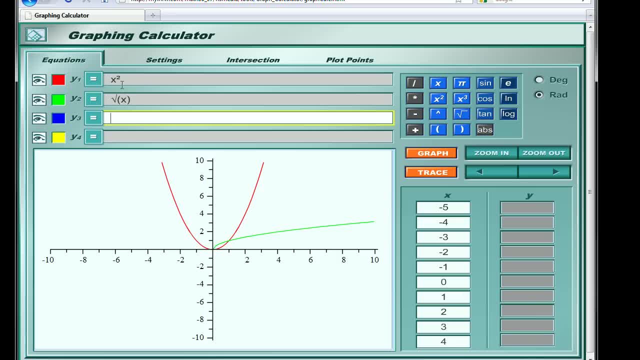 I'm going to scale the graphs and I'm going to shift them, So that's x squared. So let's just focus on the x squared and see what happens when we scale it, And then I'll do it with the radical sign as well. 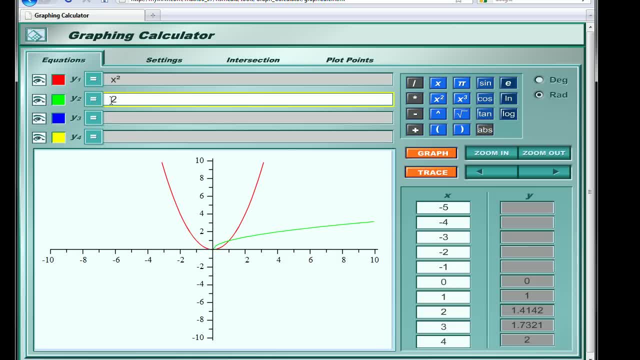 This will really work for anything. Let's see what happens when you get 2 times x squared- No, not 2 squared, 2 times x squared, And let's do another one that is 1.5 times x squared. Let's graph these right there. 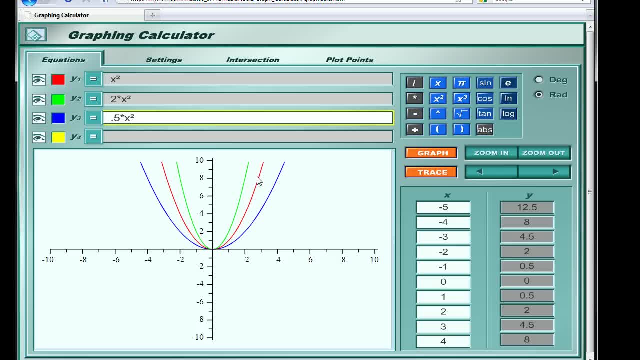 So x squared. So notice our regular x squared is just in red. If we scale it by 2, it's still a parabola with the vertex at the same place, But we go up faster in both directions. And if we have 0.5 times x squared we still have a. 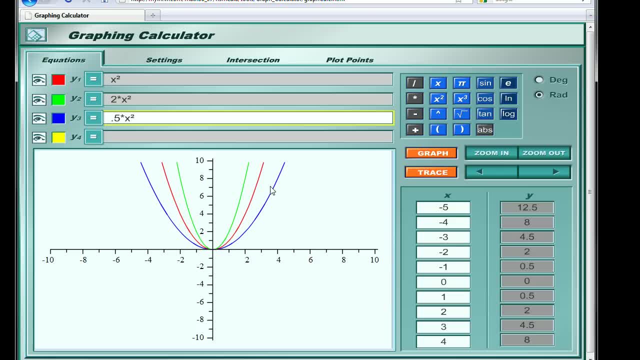 parabola, but we go up a little bit slower. We have a wider opening u because our scaling factor is lower than 1. So that's how you kind of decide how wide or how narrow the opening of our parabola is. 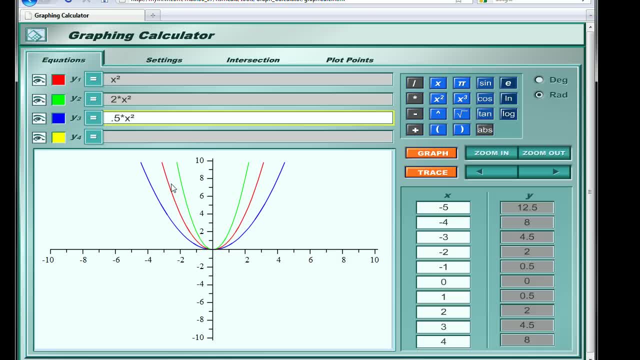 And then if you want to shift it to the left or the right- and I want you to think about why this is So, that's x squared. Let's say I want to just take the graph of x squared and I want to shift it. 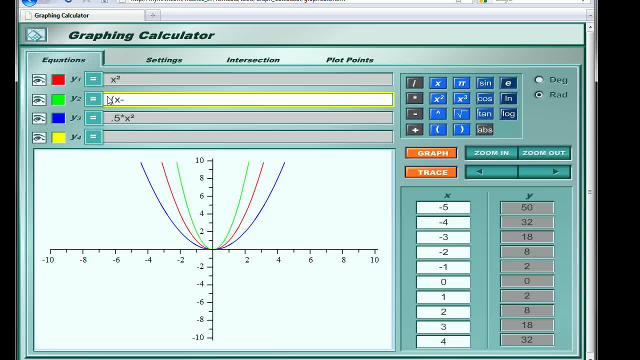 4 to the right. What I do is I say x minus 4 squared. And if I want to shift it, 2 to the left, x plus 2 squared. what do we get? Notice, it did exactly what I said. 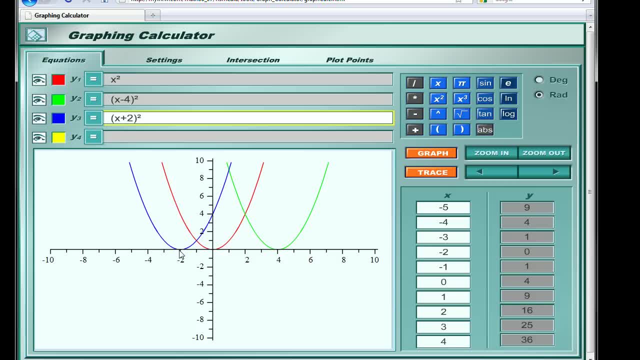 x minus 4 squared was shifted- 4 to the right. x plus 2 squared was shifted- 2 to the left. And it might be unintuitive at first, this shifting that I'm talking about. But really think about what's happening. 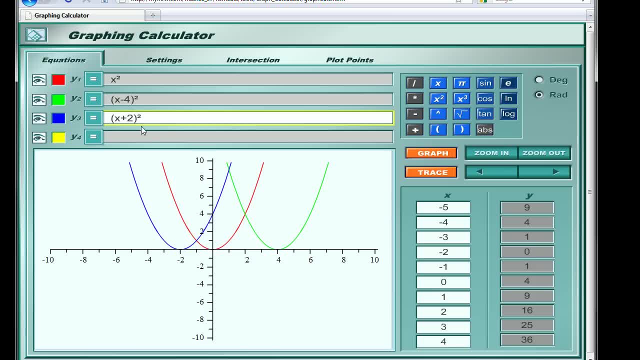 Over here the vertex is where x is equal to 0, when you get 0 squared up here. Now over here the vertex is when x is equal to 4.. But when x is equal to 4, you stick 4 in here. you get 4. 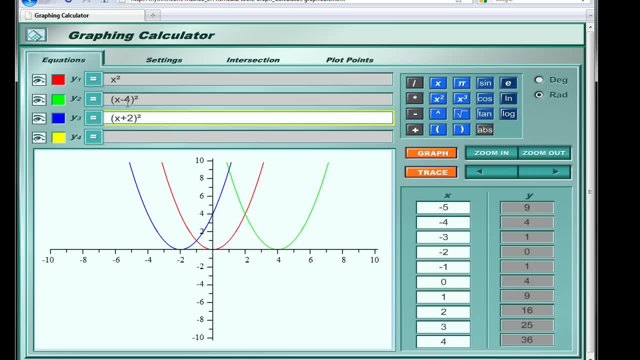 minus 4.. So you're still squaring 0.. 4 minus 4 is 0, and that's what you're squaring Over here. when x is equal to negative 2, negative 2 plus 2, you are squaring 0.. 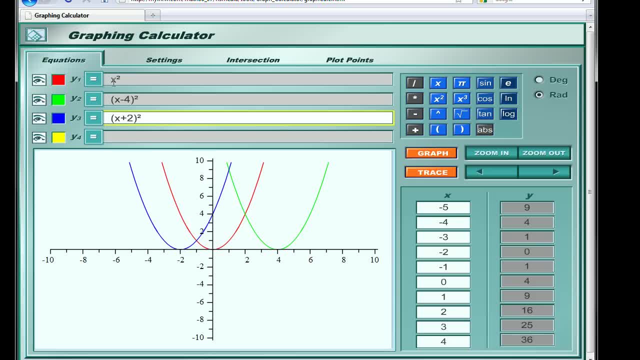 So, in other words, whatever you're squaring, you're squaring 0.. So you're squaring that at 0 is equivalent to 4 here, or 4 is equivalent to 0, and negative 2 is equivalent to 0 over there. 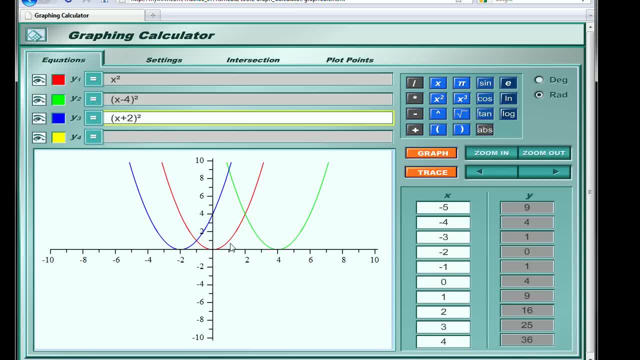 So I want you to think about it a little bit. Another way you could think about it: when x is equal to 1, we're at this point of the red parabola- but when x is equal to 5, on the green parabola, you have 5 minus 4.. 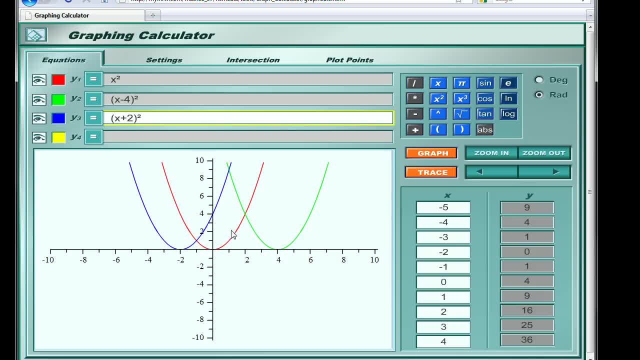 Inside of the parentheses you have a 1, just like x is equal to 1 over here up here. So you're at the same point in the parabola. So I want you to think about that a little bit. It might be a little non-intuitive that you should. 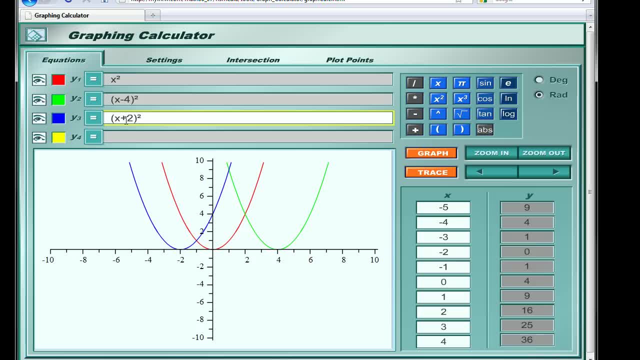 say, minus 4 to shift to the right and plus 2 to shift to the left, but it actually makes a lot of sense. Now, the other interesting thing is to shift things up and down, and that's actually pretty straightforward. You want to shift this curve up. 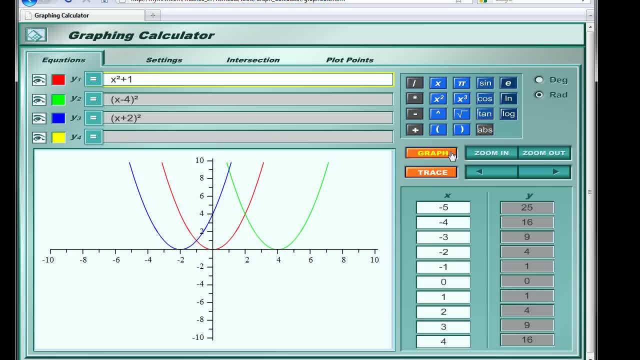 Let's say you want to shift the red curve up a little bit. You do x squared plus 1.. Notice it got shifted up. If you want this green curve to be shifted down by 5, you put a minus 5 right there. 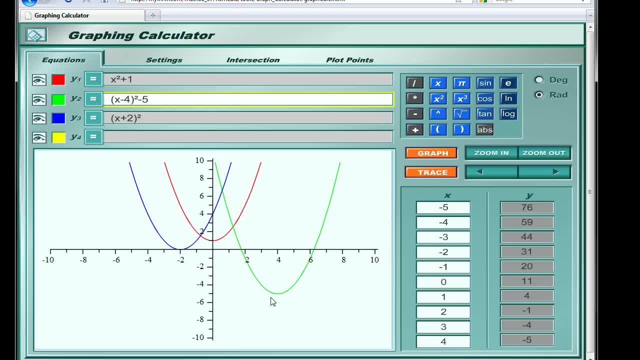 And then you graph it and it got shifted down by 5.. If you want it to be, We'll open up a little wider than that. maybe scale it down a little bit. Scale it down, let's say 0.5 times that. 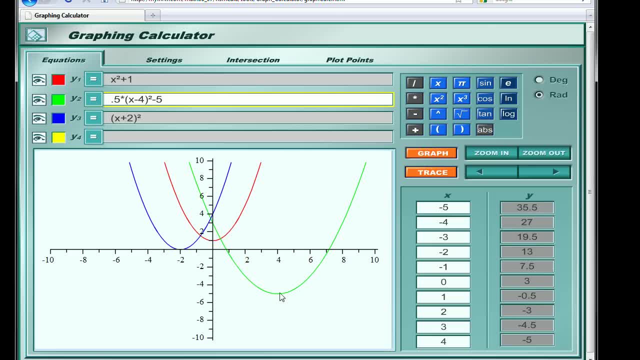 So now the green curve will be scaled down and it opens slower, it has a wider opening, And the same idea can be done with the principal square roots. so let me do that, Let me do the same idea, And the same idea actually can be done with any function. 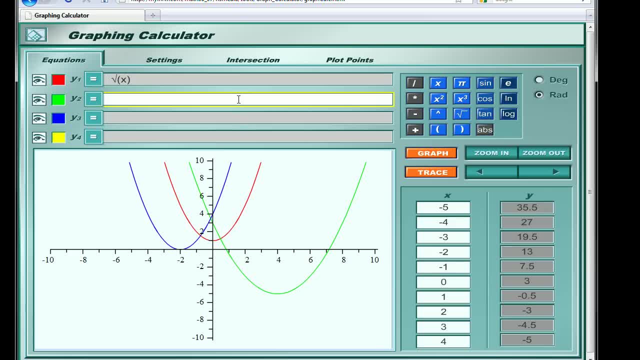 So let's do the square root of x And let's In green, let's do the square root of x, let's say minus 5. So we're shifting it over to the right by 5. And then let's have the square root of x plus 4.. 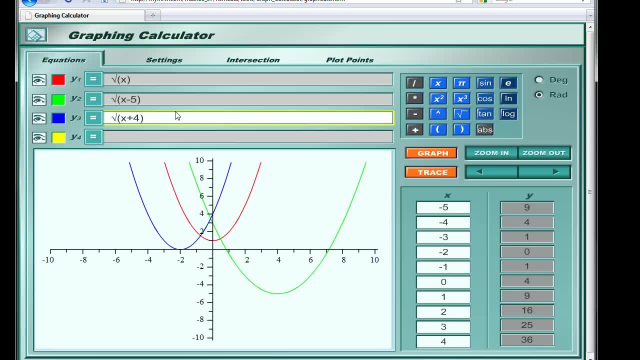 So we're going to shift it to the left by 4, and let's shift it down by 3.. And so let's graph all of these, So the square root of x, Then I have the square root of x minus 5.. 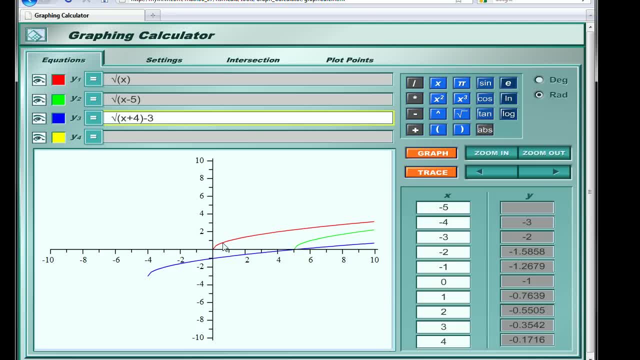 Notice: it's the exact same thing as the square root of x, but I shifted it to the right by 5.. When x is equal to 5, I have a 0 under the radical sign, Same thing as the square root of 0.. 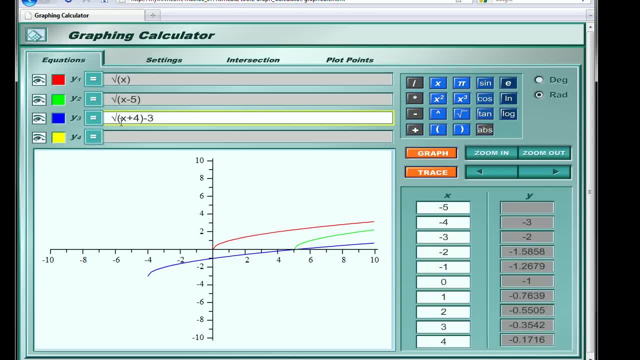 So this point is equivalent to that point. Now, when I have the square root of x plus 4, I've shifted it over to the left by 4.. When x is negative 4, I have a 0 under the radical sign. 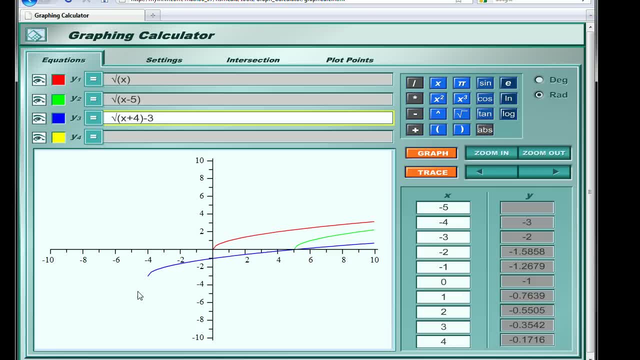 So this point is equivalent to that point. And then I subtracted 3,, which also shifted it down 3.. So this is my starting point. If I want this blue square root to open up slower, so it'll be a little bit narrower. I would scale it down. 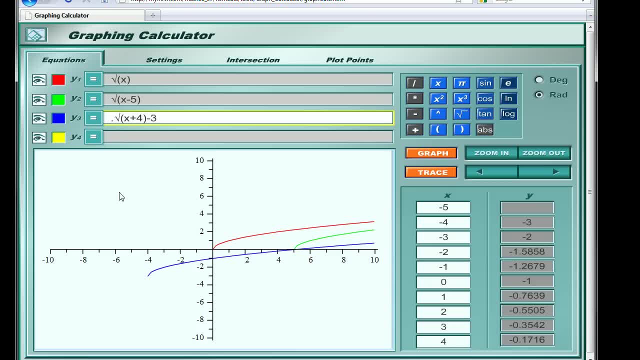 So here putting a low number will scale it down and make it more narrow because we're opening along the x-axis. So let me do that And let me make this green one, let me open up wider. So let me say it's 3 times the square root of x minus 5.. 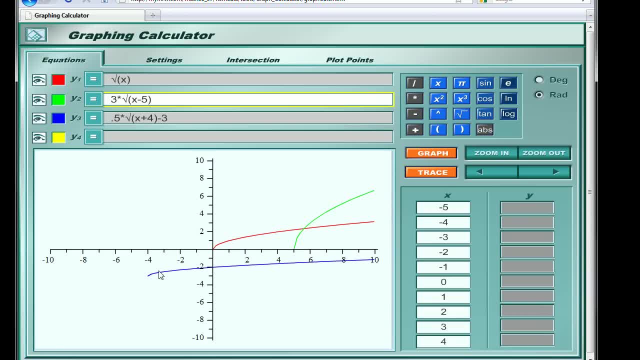 So let's graph all of these. So notice, this blue one now opens up more narrow, and this green one now opens up a lot faster. It's scaled up. Then we could shift that one up a little bit by 4. And then we graph it. 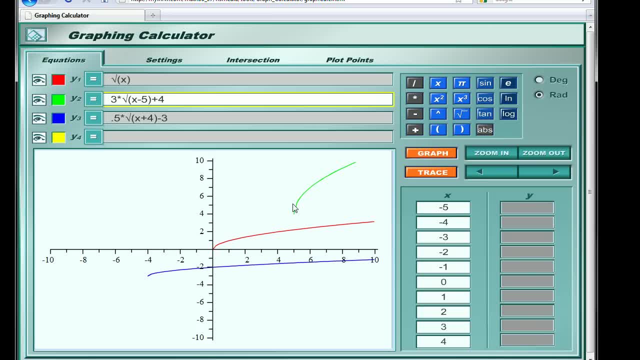 And there you go And notice that when we graph these, it's not a sideways parabola, because we're talking about the principal square root And if you did the plus or minus square root, it actually wouldn't even be a valid function because you